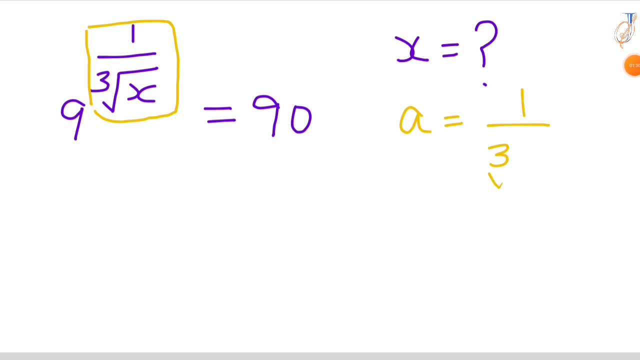 a equal to 1 by cube root of x, Then our equation turns into 9 power a that is equal to 90.. If you divide both sides by 9, then right hand side you will get 10.. In the left hand side we: 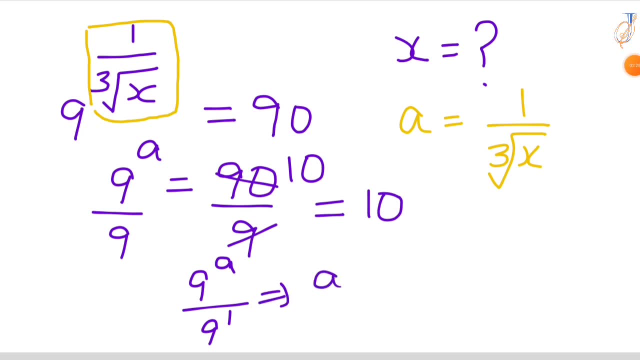 have 9 power a by 9 power 1.. It is in the form of a power m by a power n that is equal to. you can write this: a power m minus n- Same like that. you can write 9 power a minus 1 that is equal to. 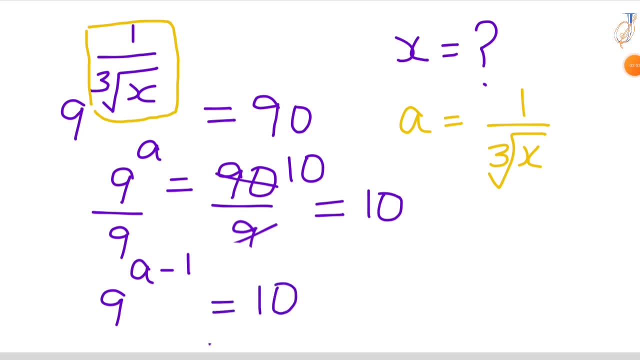 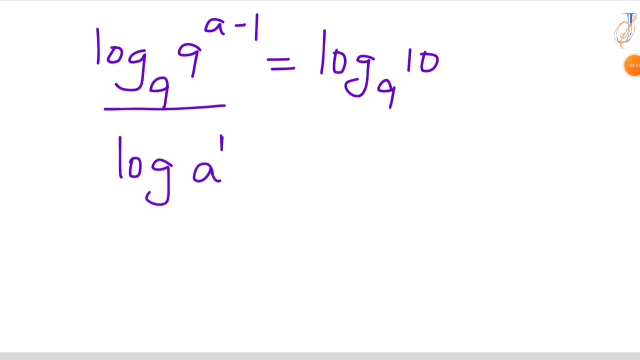 10.. Now taking the logarithm on both sides with the base 9.. Log 9: power a minus 1 base 9. that is equal to log 10, base 9.. The left hand side. it is in the form of log of a power m. We can write this: m times log a, Then our equation becomes a minus 1. 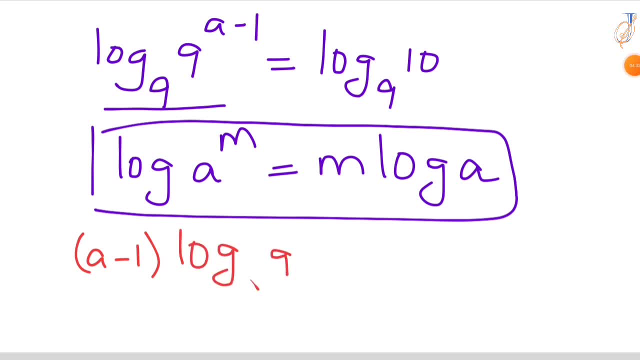 log 9 base 9, that is equal to log 10 base 9.. a minus 1 times 1.. Since log 9 base 9, the value is 1.. So here comes 1, that is equal to log 10 base 9.. LHS, it becomes: 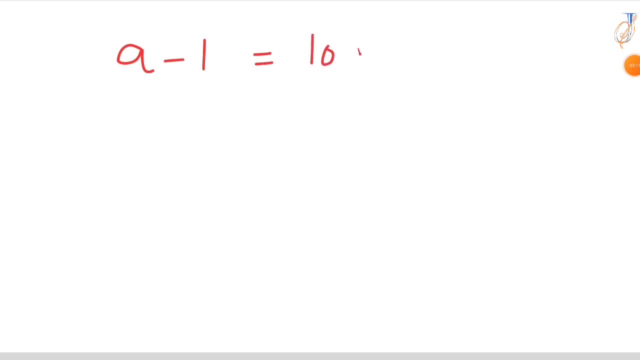 a minus 1.. Then RHS, we have log 10 base 9. This in LHS, this minus 1. if we send to opposite side then become plus 1. So that is a equal to 1 plus log 10 base 9.. We consider a equal to. 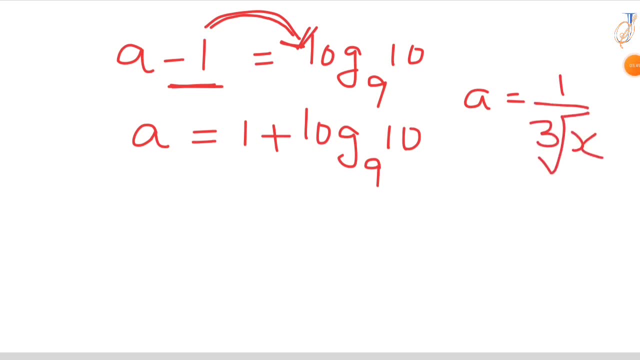 1 by cube root of x. You take that one, So 1 by cube root of x. that is equal to 1 plus log 10 base 9.. Cube root of x is 1 by 1 plus log 10 base 9.. If you do cube root on both sides, then this cube and 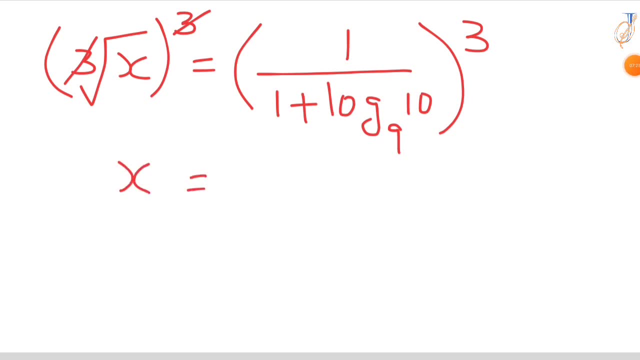 cube root gets cancelled, Then you have left only x. that is equal to 1 by 1 plus log 10 base 9 whole cube. Now if you know this log 10 base 9 value, then easily you can tell the x value. So that is why first find log 10 base 9 value, Log 10 base 9. it is in the form of log a. 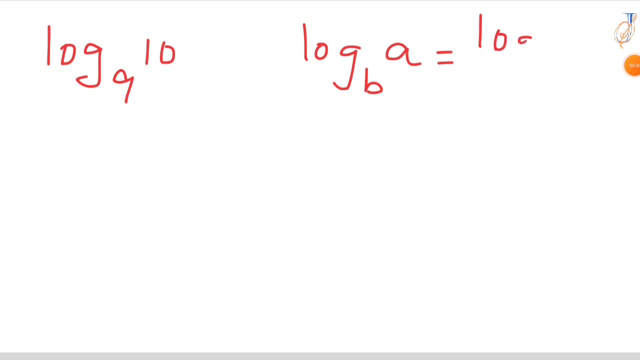 base b. We can write this log a by log b, equal to. you have to write log 10 by log 9.. And we know that log 10 value is equal to 1 by 1 plus log 10 base 9.. So if we see here we have 1 by 1 plus log 10 base 9.. 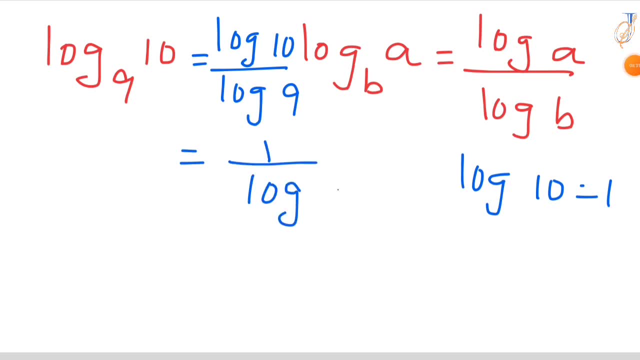 is 1, so 1 by log 9. we also know that log 9, the value is 0.954. 1 by log 9, the value is 0.954. if you do division here, 1 by 0.954, the value is 1.049. so log 10, base 9, the value is 1.049. 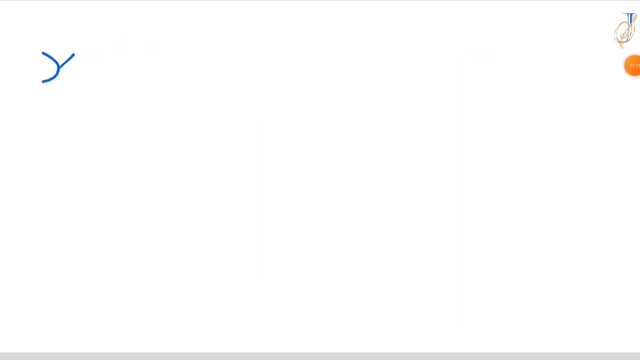 substitute in our x value. x value is 1 by 1 plus log 10 base 9. so what is log 10 base 9? value 1.049, 1.049. this is whole cube. so then x equal to 1 by 2.049 whole cube. 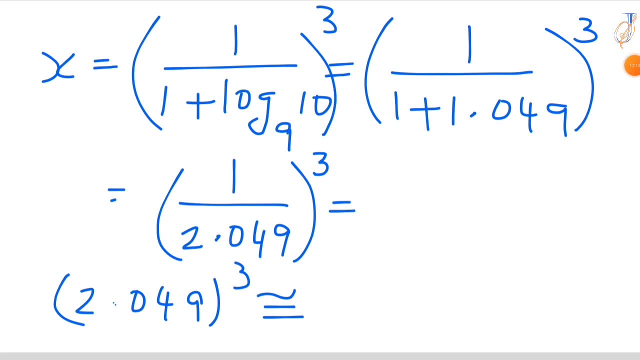 2.049 is nearly. the value is 8 point something that is 337. so the x value is 1 by 8.337. so if you do calculation, then you will get. this x value is nearly equal to 0.1199. that is the x value. thank you for watching this solution. 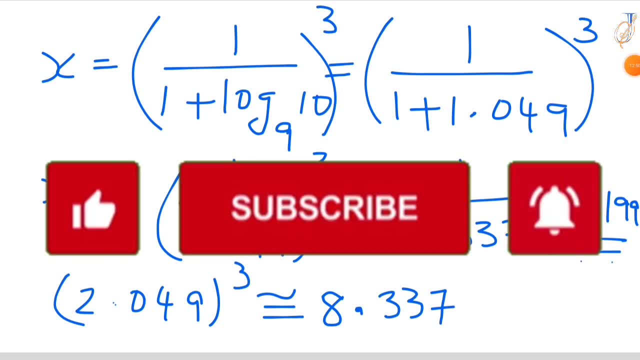 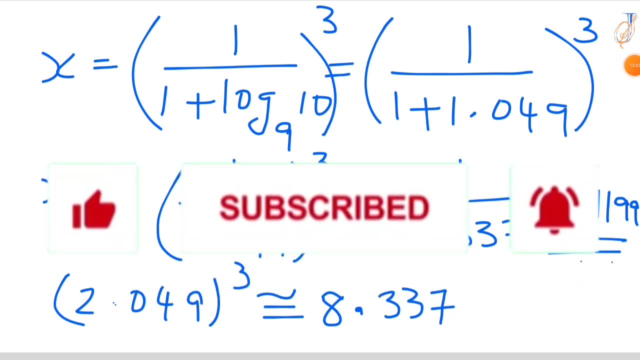 if you found it helpful and want to see more explanation and tips for olympic problem, make sure to subscribe my channel. your support means a lot and helps me continue creating content. see you in the next video.